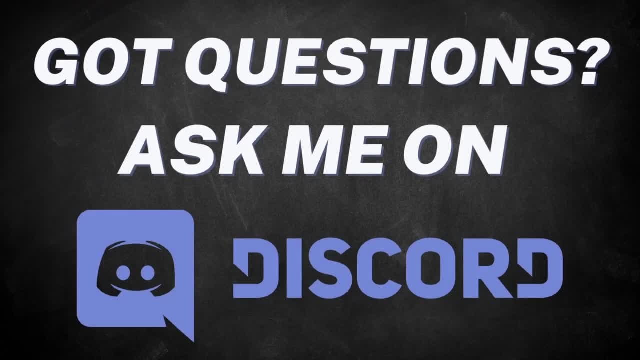 I'll also provide a link for you to join my Discord server, where you can discuss web development with other students and you can ask questions that I can answer and receive help from other viewers too. I look forward to seeing you there. The starter code for today is at the GitHub. 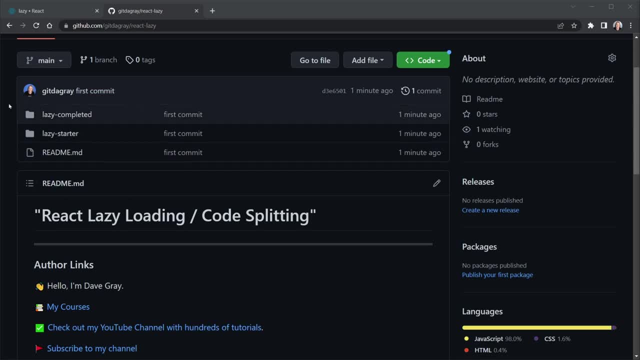 link in the description and there will be a starter directory and a completed directory. Both directories have a working sample React app, but only the completed directory has code splitting applied with React lazy. Let's look at our example React app. You can see we have. 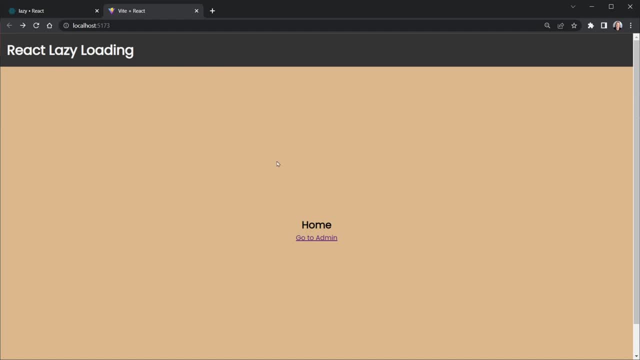 a bar at the top that says React- lazy loading, and in the middle we just have a word home, and then there's a link that says go to admin, so we can go to an admin page. Now, for today's purposes, we're going to have to pretend that this link is only visible to people that would have an 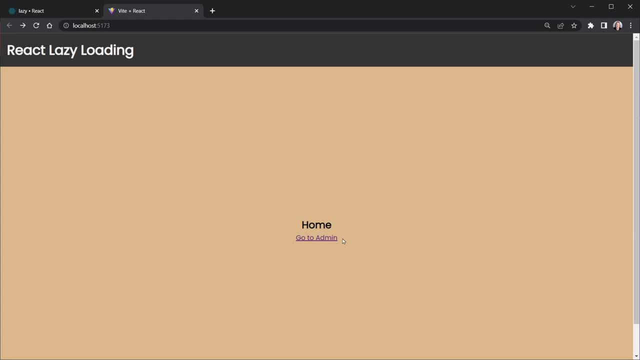 admin role. I did not set up roles and all of those things for this tutorial because we can just say, okay, only admins can see this link, and if they can see this link, then they can click it and go to an admin page as well, and it's a really simple page. Now I did put like a hundred 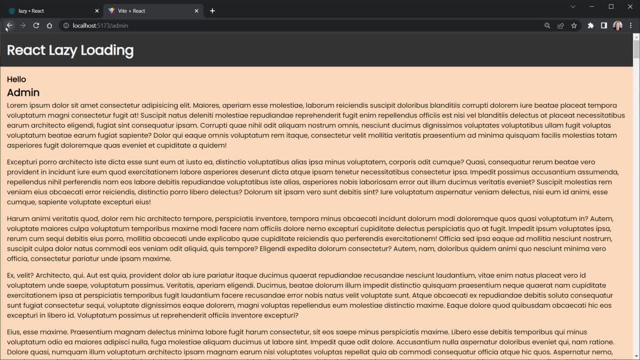 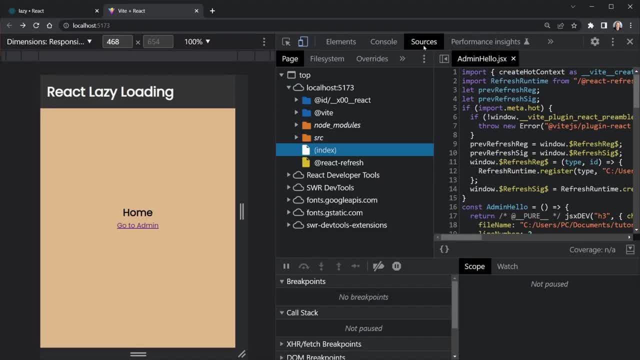 paragraphs, just so you can see what's going on. I'm going to go to the admin page and I'm going to set it up, just so. it had a lot of content with a lot of words, but besides that very simple page, Now I want to open DevTools and what we should look at. I'm at the sources tab in DevTools here. 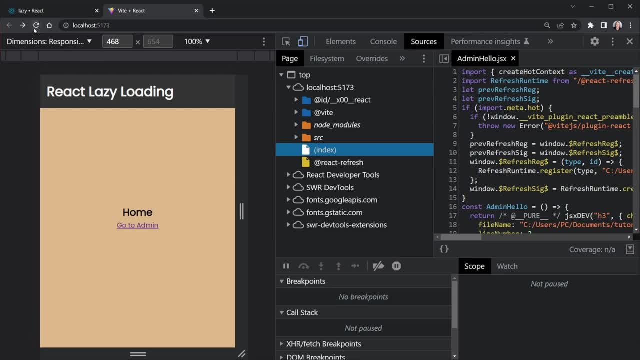 in Chrome When we reload- and when we do reload today- we will right click on the reload and we'll choose empty cache and a hard reload. Now, when we do this, we want to look in the source directory to see all of the components that have loaded. So here we have the main page and the main page. 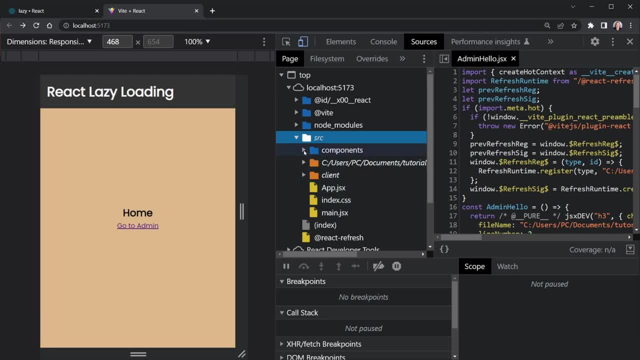 And the app page and there's our index css. Now, if we open up the components directory here, we can see there's a layout component, because we're using React Router. There's a home component, a header, and then there's an admin and an admin. hello, So two specific components that you could. 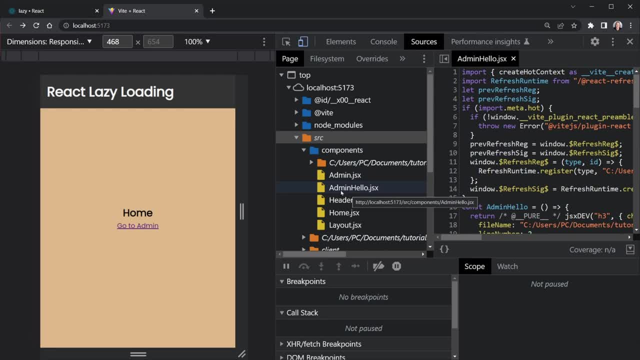 only use if you're an admin. The rest of the users of our app would not be able to use these components. And then there's also some skeleton loaders in here, I believe as well, and we may see those, But over the course of this tutorial we're going to be looking at a lot of components that 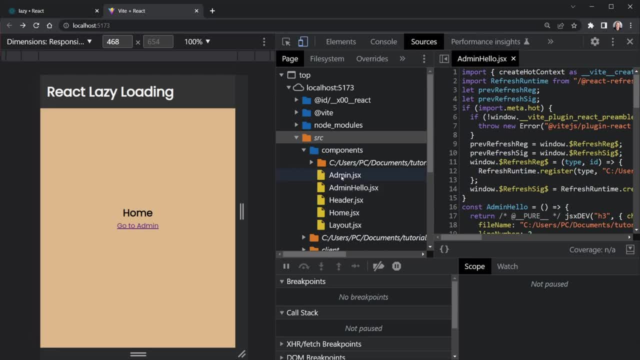 we want to pay attention to. So, overall, the main thing we want to pay attention to is the admin hello and just the admin component overall, because we're loading this in no matter who loads our web app. But we don't really need to do that. We only need to load in the admin components. if an admin 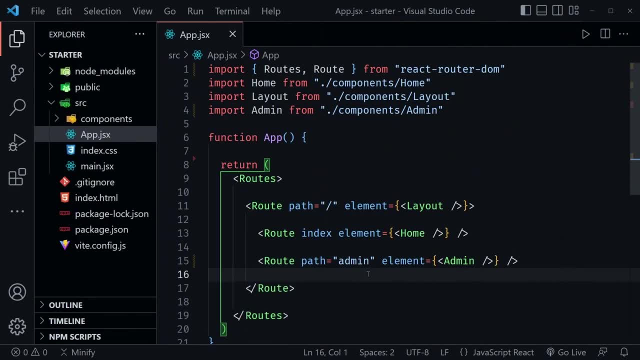 is going to use our web app. So now I'm in VS Code and let's take a quick look at this starter code. Now I am using React Router today. If you're not familiar with that, I have a tutorial for React Router on my channel And then, in the background, I have a tutorial for React Router on my channel. 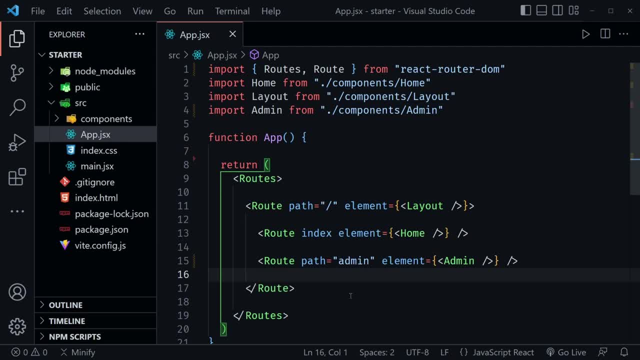 But in the very recent past here I have completed tutorials on skeleton loading components and also on React Suspense, And we'll be using both of those today. So if you want to dive deeper, look for those on my channel. Now let's look at this code. This uses React Router. I put the main React. 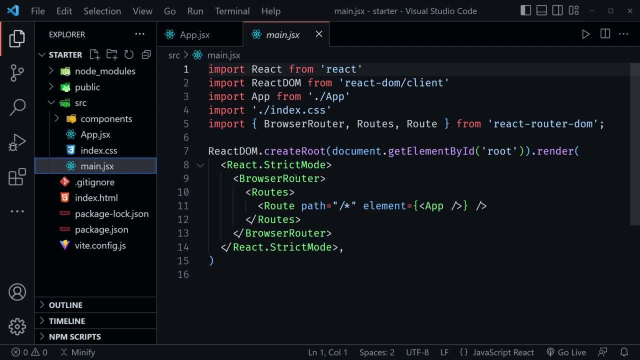 Router code in the mainjsx here And that's what we have, because it is a Vite application that we used here instead of Create React App. So we have Browser Router from React Router and then Route Routes, And then I take my single route and it has the slash and the asterisk so we could nest. 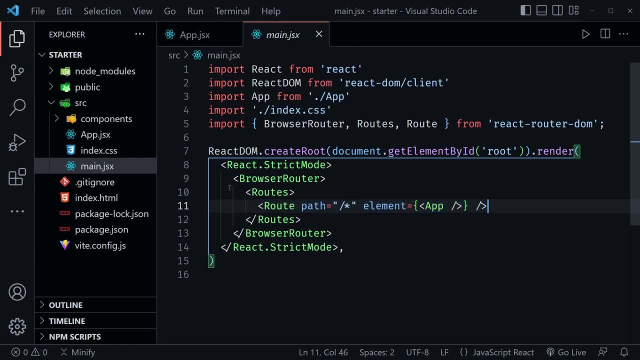 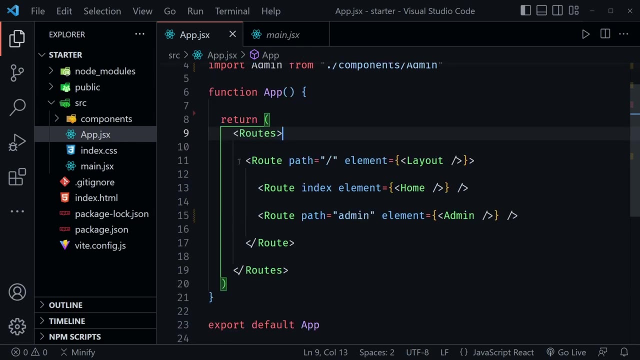 routes and send to the app, And I like to put all of that here in the mainjsx. If you used Create React App, your main would be indexed, But either way, that's where I like to put that. Then when I go to the app component, I just have everything inside of routes. Now you can see I have my main. 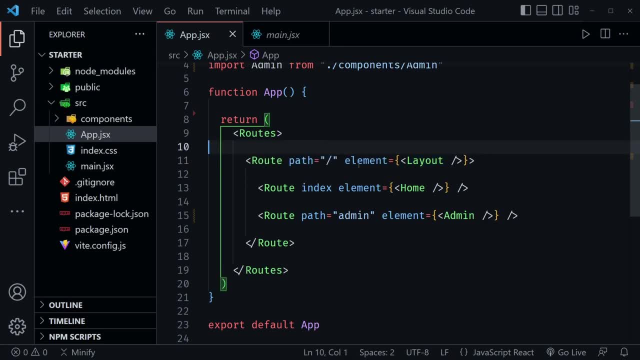 route with the slash, So really everything catches here And that's where we use this layout And that layout component brings in the header and things. So I'm explaining React Router. You may already know that, But if you don't, I'm just giving you a quick overview. Now here's our index route. 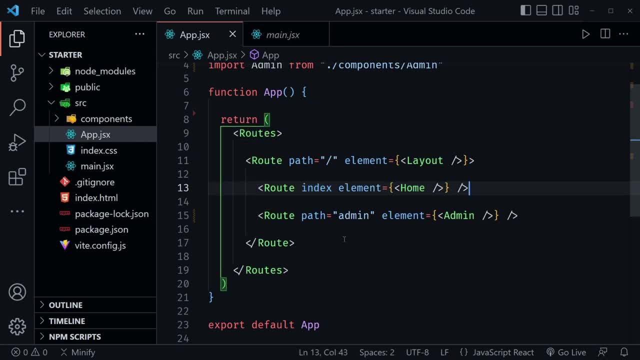 that goes to our home, So that loads immediately. And then there's the path admin, So it would be slash admin And that's what loads the admin component. So only if we could see that link as an admin would we even be able to access this component. And that's the point: today We don't. 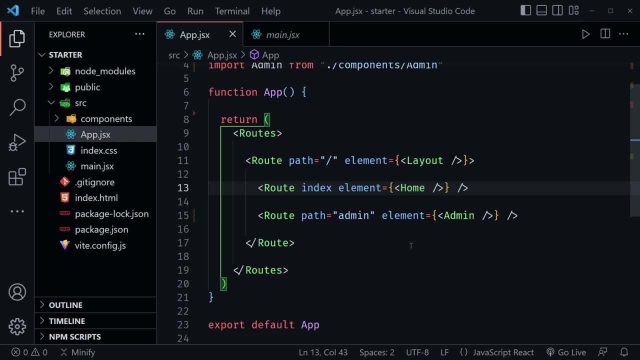 really need to load any of the JavaScript associated with React Router, So we just need to load the admin components, Unless we have an admin that can use those components, And the problem we currently have is we're sending all of our JavaScript, including the JavaScript for. 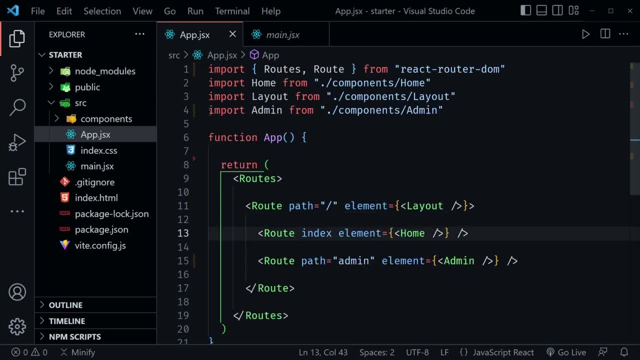 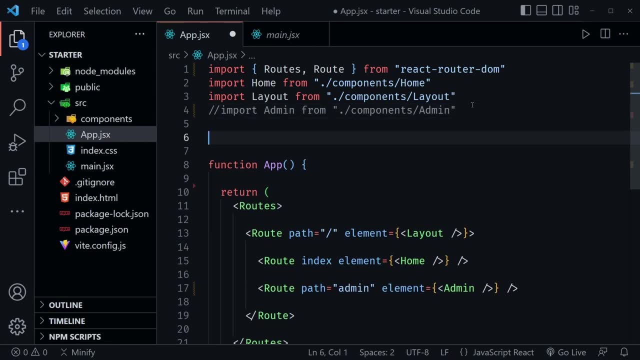 those admin components. So let's fix that And we'll start here at the top. I'm going to comment out our import of admin. Instead, I will come down just below and I will import. Now I'm going to choose lazy from React And there you can see, we have that now And instead. 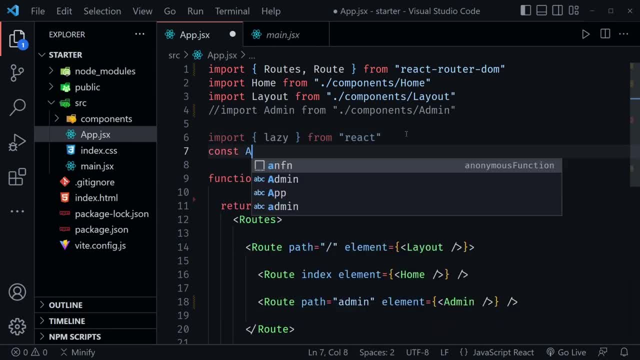 I'll define admin underneath And I'll say const admin And set this equal to lazy, Which takes a function, And then inside of this function we will import, And here we essentially specify what we did above. So it's dot components or dot slash components, slash admin. So I'll just copy this: 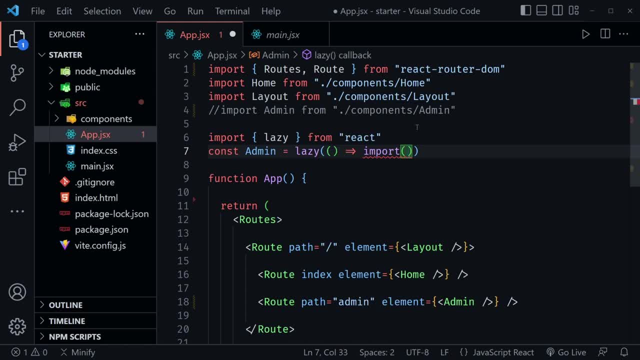 And I'll paste it right here inside of the import. Oh, it does need to be inside of quotes as well, So I'll just put single quotes There. we go And save And now we can lazy load this component. But it's not quite that easy. We actually need to wrap it. 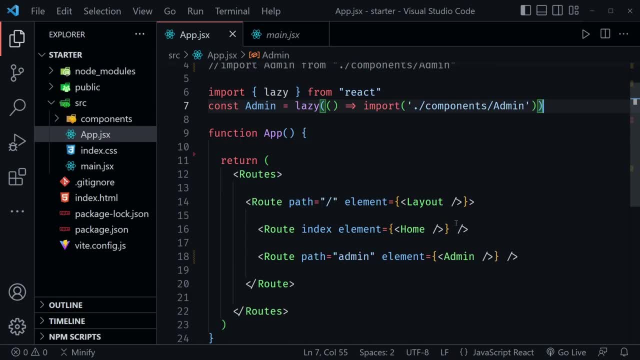 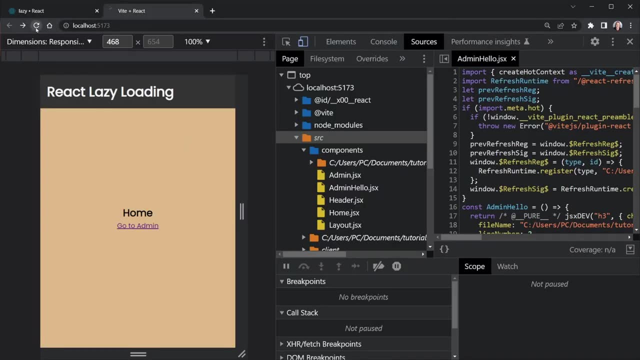 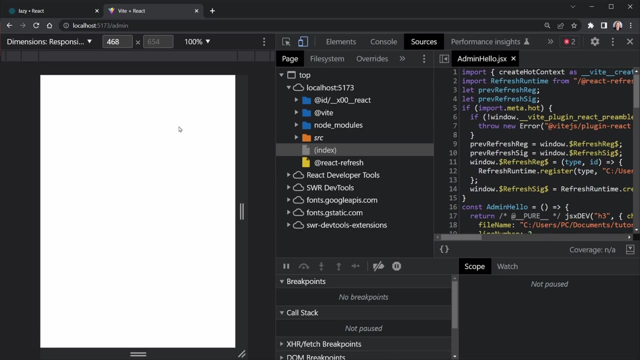 in some things as well. So we have our admin here And if we go to our application- So let me drag this over- Go back to our application And I can reload this And we should get the changes. But if I try to go to admin right now, It doesn't work. So we're not quite ready yet And that's because 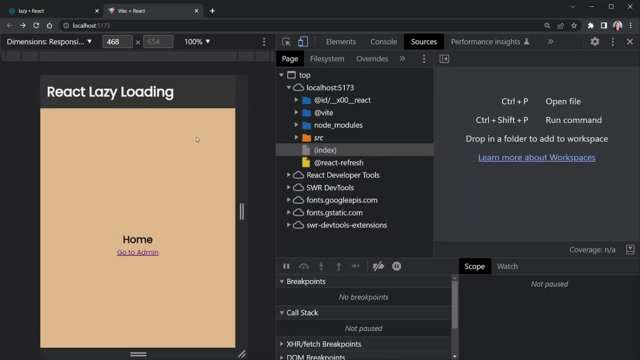 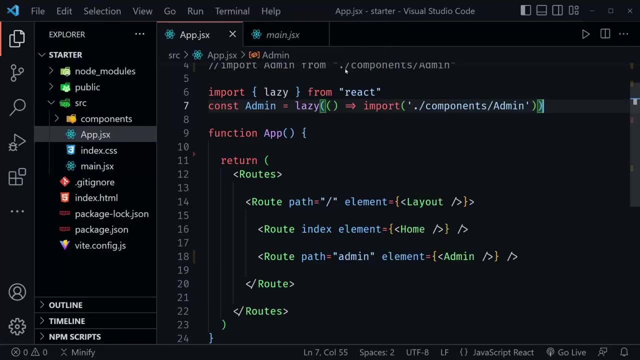 we need to do things with react lazy And I'll reload here And we're fine. now, When we reload things with react lazy, We also need to use react suspense. It's a requirement. And we also have another requirement And that is to use default exports. So, for example, in our admin component. 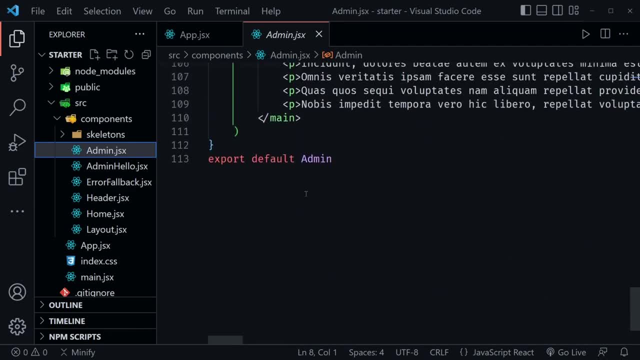 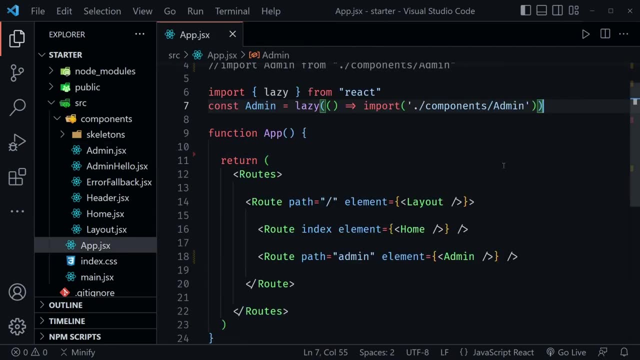 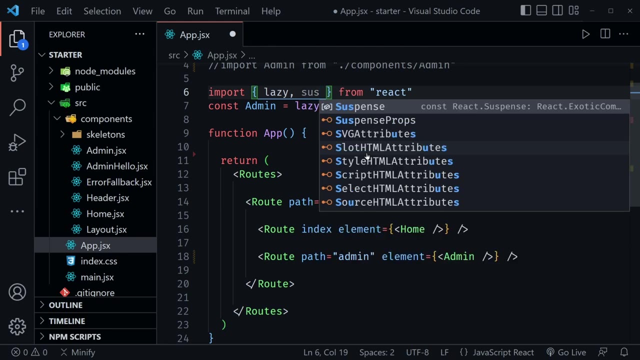 And you can see I have the 100 paragraphs here Rather large. But when I get to the bottom I do have the export default for admin, And that's what lazy expects. So we need to use the default exports And then we need to use suspense from react as well. So let me import that here at the 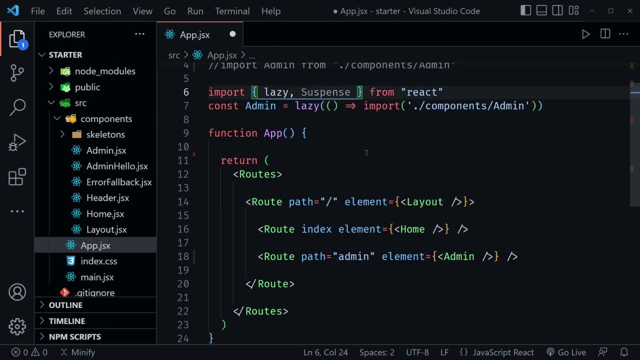 top there. I saw it in the list And now we can use suspense. And now to use suspense Instead of wrapping it around, a route. You cannot do that in react router, We need to put it right here inside of the element equals. So I'm just going to come down to add some extra lines here And then we'll. 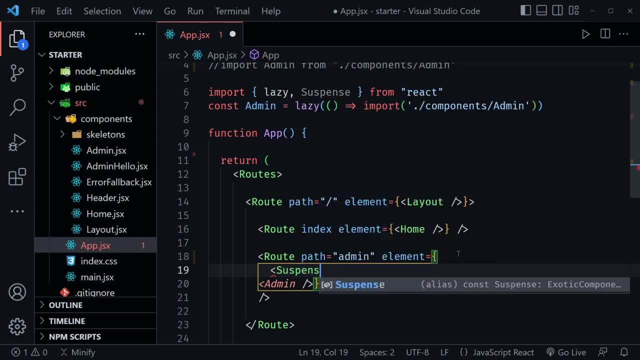 wrap this admin component in suspense, So let's add suspense Now. suspense has a fallback And we'll set that equal to our skeleton admin component that I already created. And, once again, if you're interested in learning how to create skeleton loading components, I have a separate. 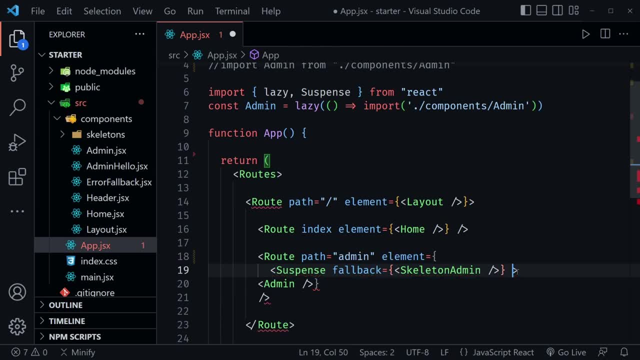 tutorial on those as well. Whoops, I closed that out And we don't want to do that. We just want the caret there Because we need the closing suspense after admin. So here we would have the slash, There it is, And suspense, And once I save it should look a little bit better. There we go. 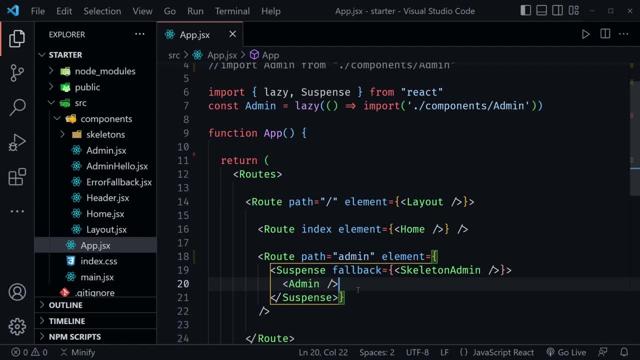 So we've wrapped admin and suspense, But what we learned in my tutorial about react suspense is that you should always use an error boundary with react suspense as well, And so we need to add react error boundary as a dependency. And then I'm going to come back and update the imports, Because we 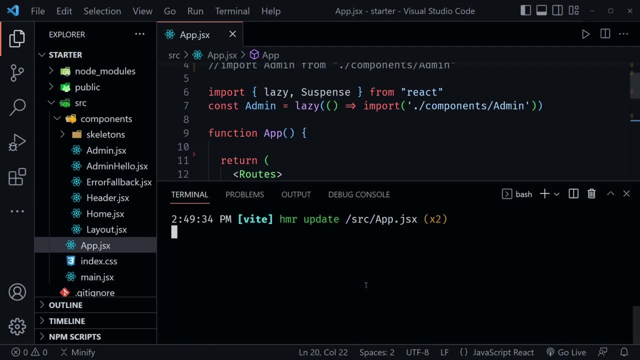 need to import that skeleton admin component as well. So I will open up the terminal here, Control C, to currently stop our dev from running. And now let's say npm i And we want react dash error, dash boundary added as a dependency. So I'll quickly add this And we could look at our package. 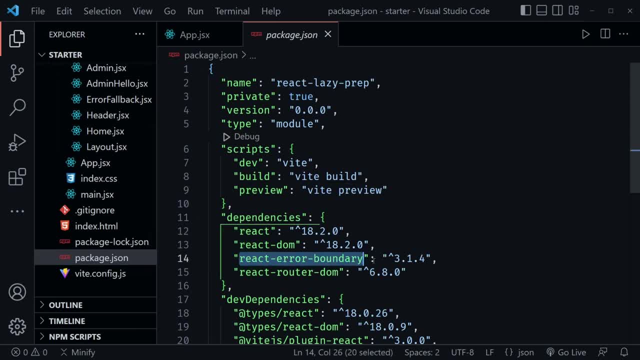 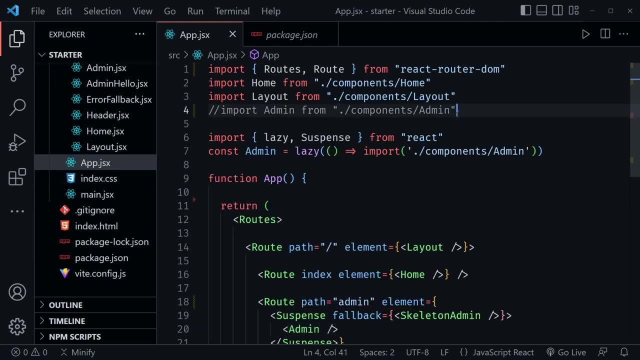 JSON Just to make sure it is there. And now we see react error: boundary has been added. Let's go back to the app now. And now let's add all of those imports that we need up here above. So I will come down a couple of lines and say: import. Now I want. 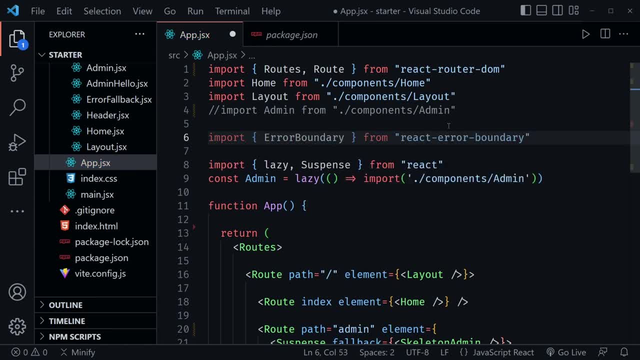 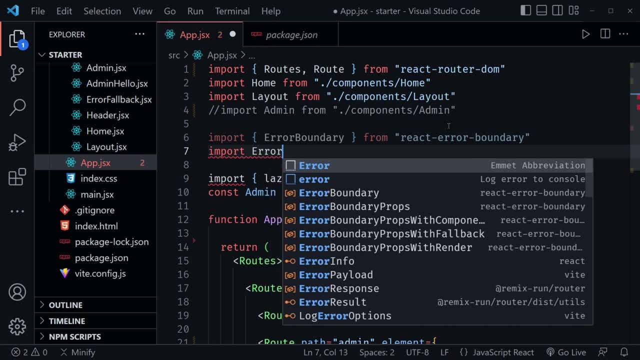 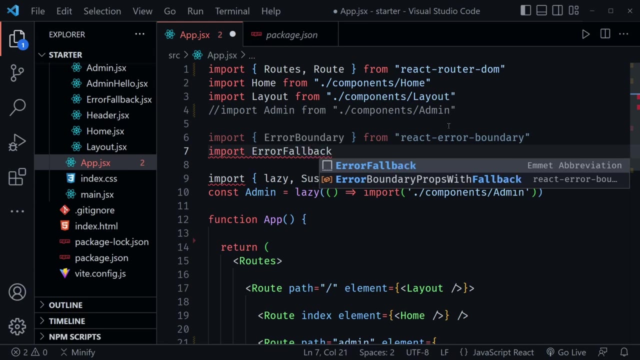 error boundary. So I'll find that in our list from react error boundary. That is correct, and then I have created an error fallback component as well and it is really from the error or react error boundary docs, and so you could learn more about that in my tutorial again. 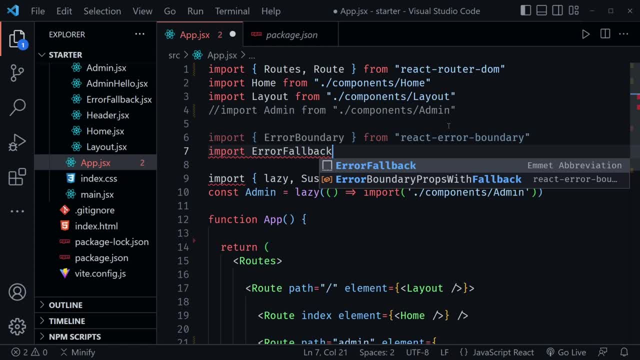 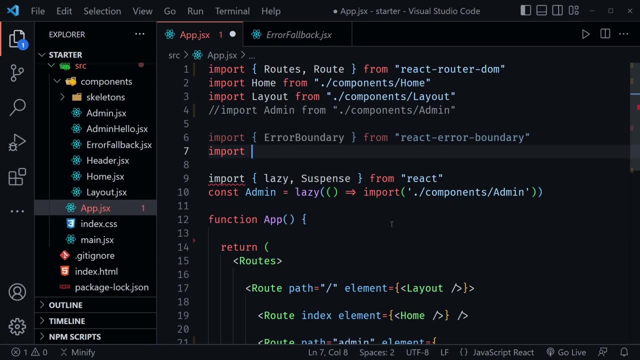 about react suspense and react error boundaries, but so this component is just called error fallback. so now go ahead. and well, that didn't work. let me find that here. do we have it in our component list? yes, there, it is right here, so we can get that from components. we want import error fallback. 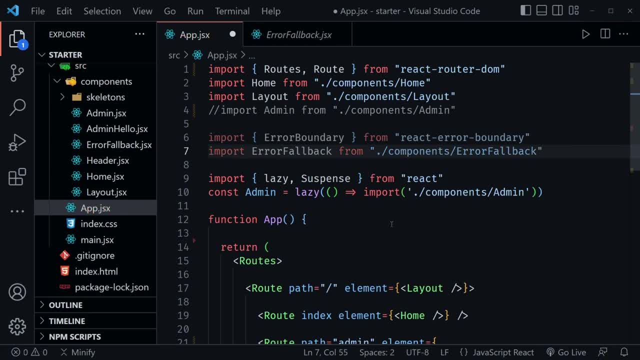 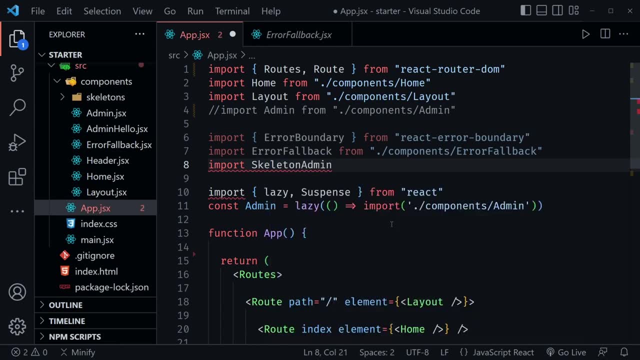 there it is in the list, I just missed it before. so we've got error, boundary error, fallback, and now I need that skeleton admin component as well. there, I see it in the list and it didn't auto complete for me. so I want from dot slash components, slash skeletons, slash skeleton admin. 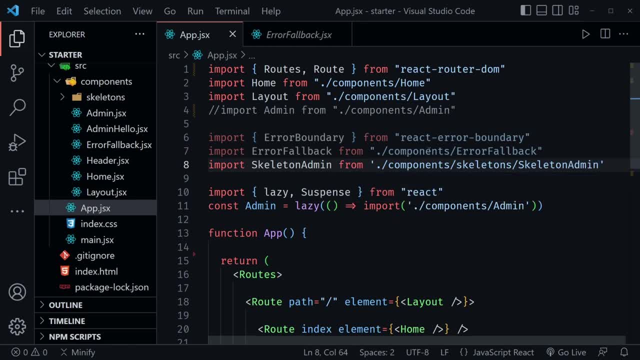 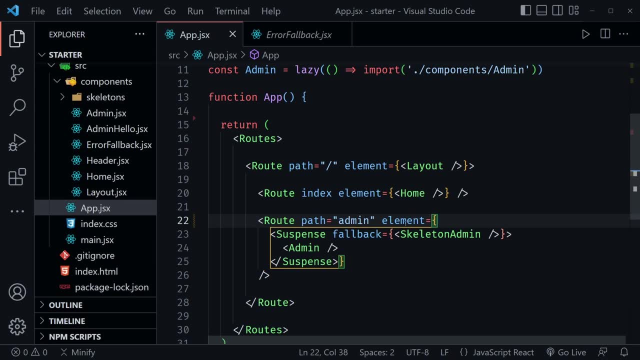 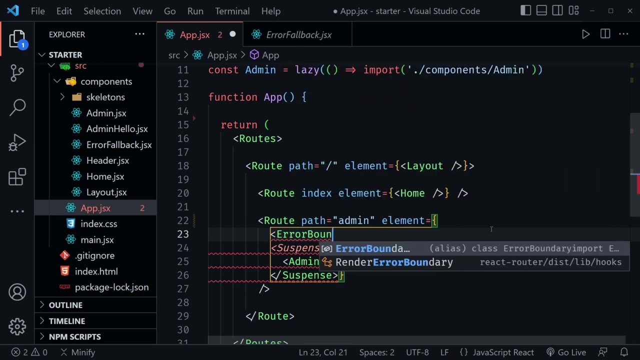 there it is. now I've got all the imports I need, but we still need to wrap our suspense in that error boundary. so once again, still within this element equals here of our route, let's add this error boundary. so we'll start off with error boundary and then error boundary has a couple of things. 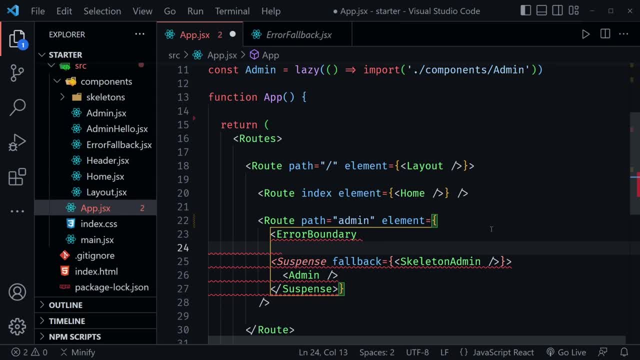 we need to add to it as well, so I'm going to add them on separate lines. the first is a fallback component and we'll set that equal to the error boundary and then we'll add this error boundary and then we'll add this error boundary error fallback component that I had imported. after that we can go ahead and add an on reset. 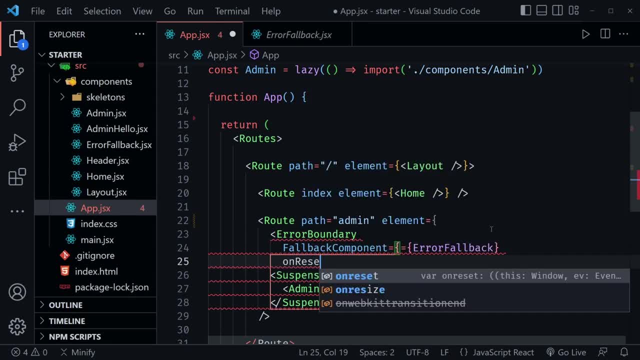 function also. so let's say, on reset equals. now, inside of this we need to provide an anonymous function and here we can provide the function or call that we want to provide. maybe this would be a set state, and that is fairly common- if we had some local state that needed to be reset. 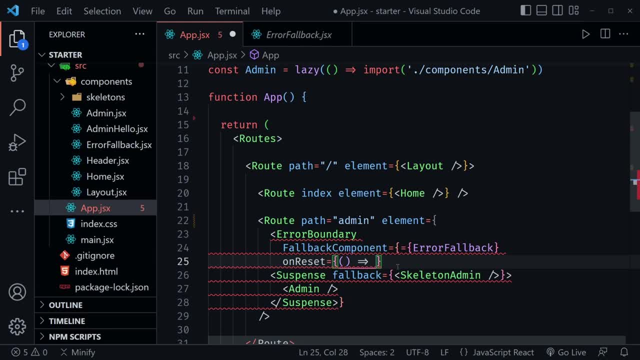 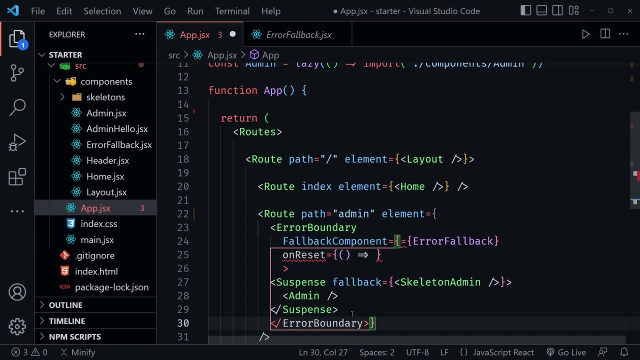 that is not what we will do right here, though I need to go ahead and close this out as well, so let me put that arrow there. that is not where we need the closing error boundary, though that is going to go. at the end of after the suspense, and before the curly bracket, there's the closing error boundary, I feel. 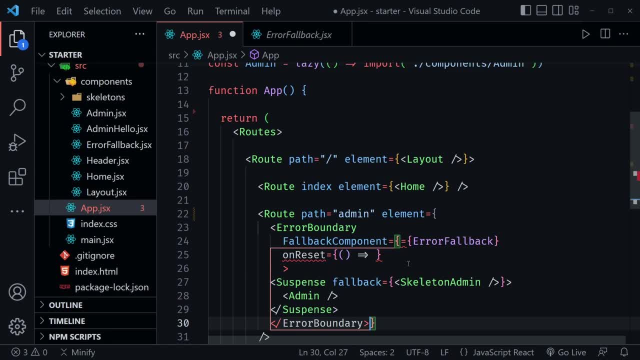 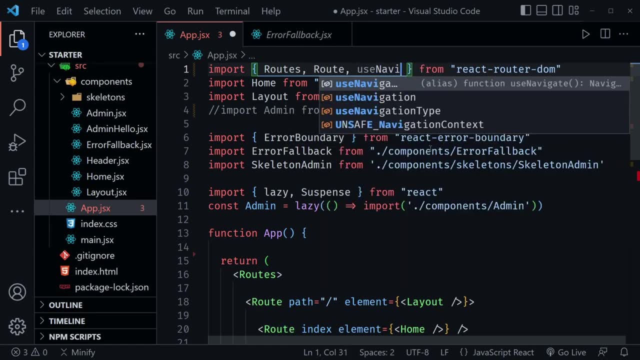 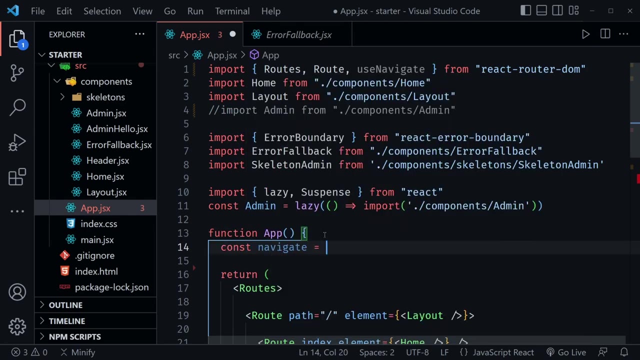 like I'm missing something else, but it's probably just what needs to go in this function. but what needs to go in the function is a navigate function, because we're using react router, so I'm going to bring in use navigate. now that I have that, I will say const navigate and set that equal to use navigate now that I have a navigate function. 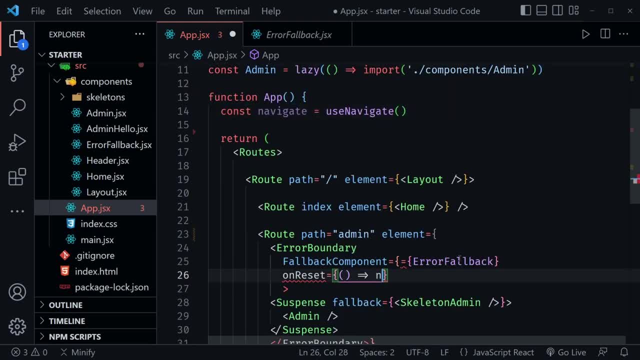 that's what I'm going to pass in here to my on reset. so I say navigate, and this will allow anybody that encounters an error. oh, and here's part of my problem here as well. so this fallback component, a couple of extra things, that looks better. so anybody that has an error, say if they. 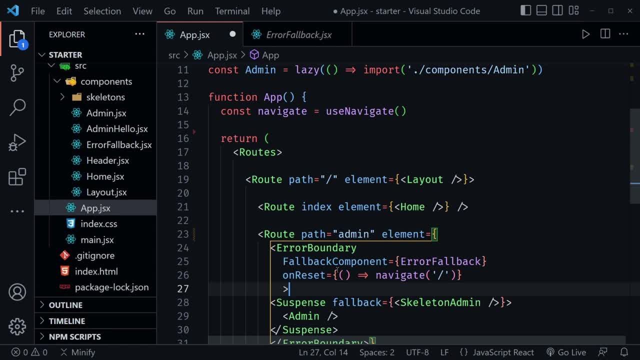 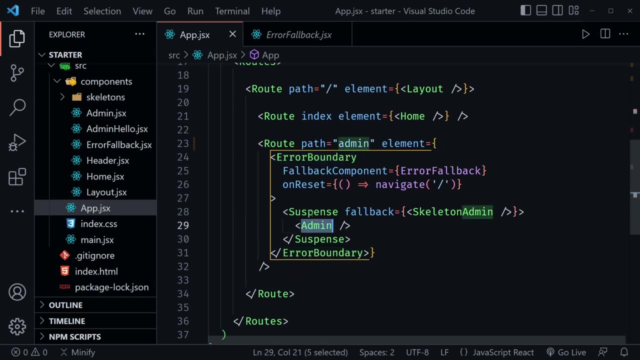 navigate to the admin page, they will get this nice error fallback component and it will give them a button that says try again. when they click that, it will navigate back to the home page, for example. so we're now wrapping our suspense in an error boundary and we have wrapped our admin component in suspense and you need to. 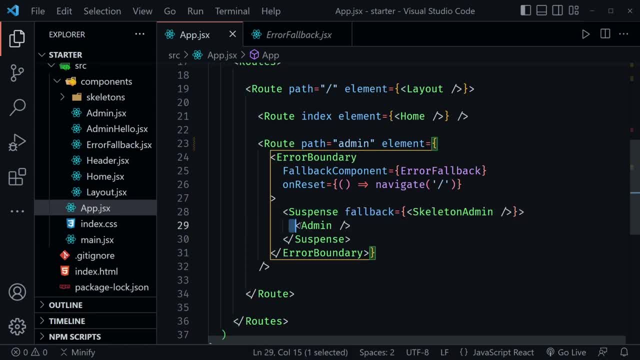 use suspense. it's required that you use it with any component that you lazy load- now i should say any component tree, because we have a nested component inside of admin that is our admin hello, we don't have to actually use lazy with it. it's going to be lazy loaded when the admin 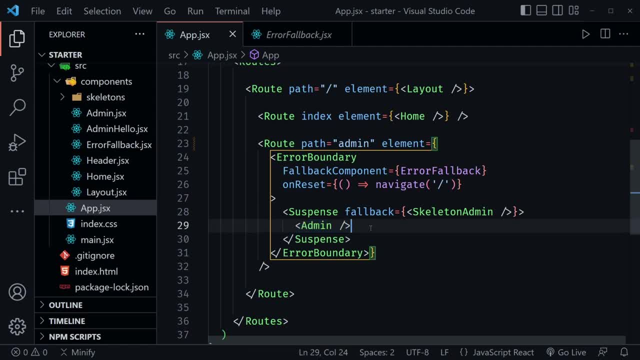 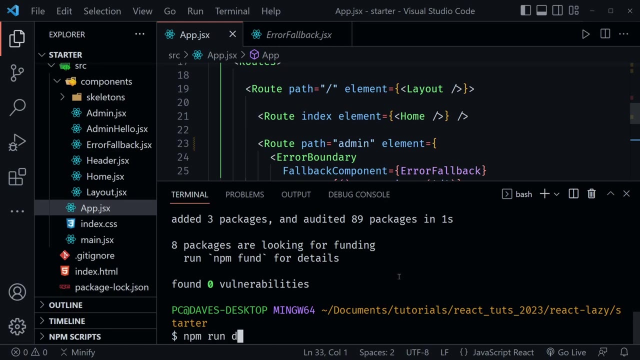 component loads, so it won't load when the hello page or our first load of our app happens. it will only load when we go to the admin page or the admin component. okay, with these changes now in place, let's go ahead and open the terminal again. we will start up our project once again with npm run dev, and now we're ready to view the project. 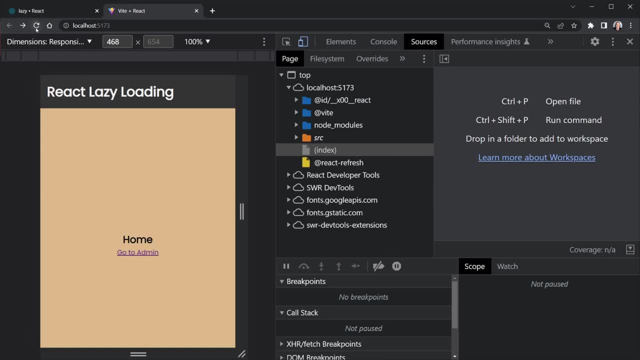 which was already in the browser, so let's just reload it over here and now. let's look at this source directory again and once we look at the source directory, we've got components here and we open this up. notice: we have no admin components. we do have the skeleton directory here and this: 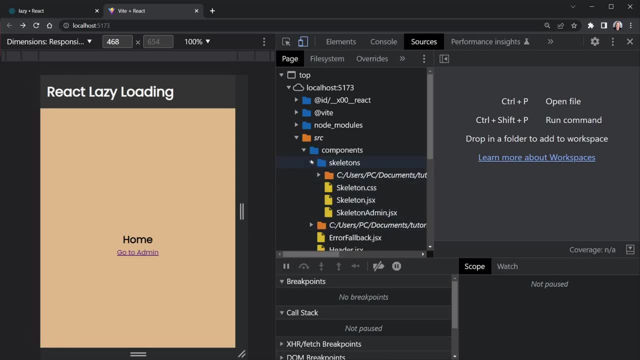 will have a skeleton for the admin, because that's what we actually like to do. so let's go ahead and open the terminal again and we'll start up our project once again. load when we're waiting on loading the admin components. that's part of react suspense. 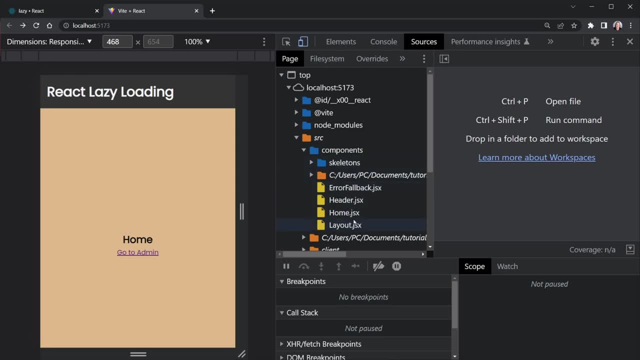 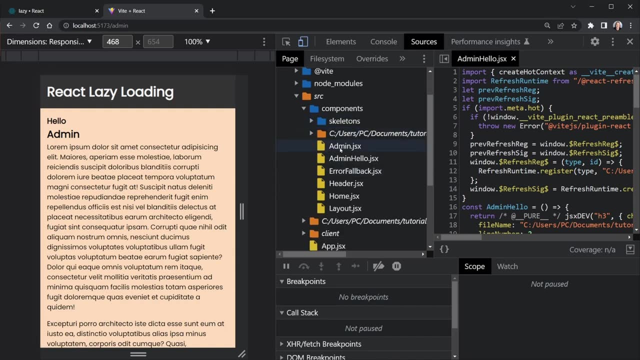 but what we have here, where we were seeing the admin and admin, hello, they did not load. so now when we go to the admin page, we see a change and now those components load. so we, lazy, loaded those. so that took a large chunk of javascript and waited to load it. it loaded it dynamically. 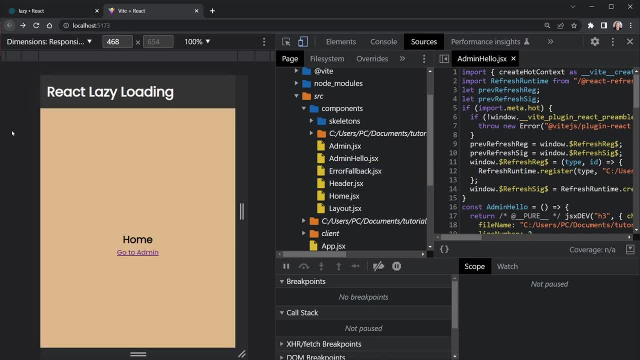 only when we went to that page. so once again, if we go back to our example, we've almost loaded up the files into a whole without lamenting and you'll see that this example is totally happening will not load, go back to our current project. so in dev mode we see all of these individual things. and if i come to the network tab, actually 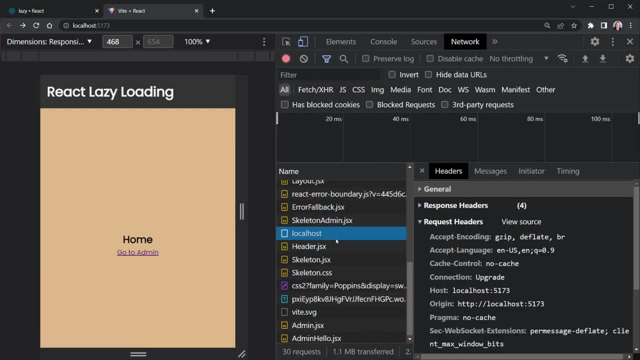 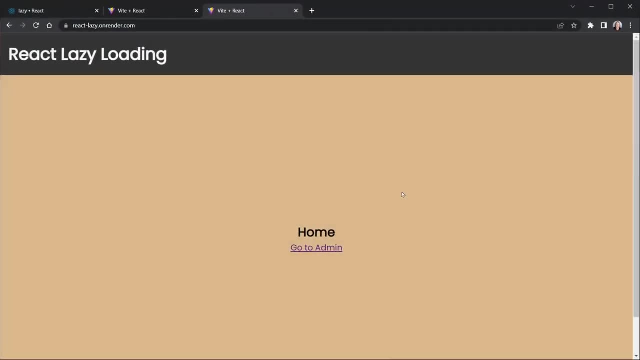 we see all kinds of things loading here, but you can see we're in localhost. this is dev mode, so i actually have this loaded up on the web. this example app, and let's look at how we get chunks of javascript when we're looking at the network tab. okay, i have this app now on rendercom, i'm going. 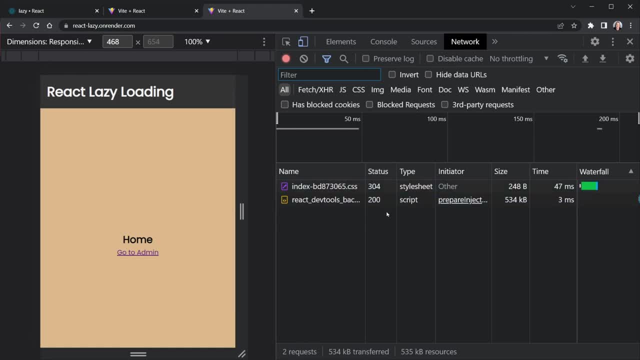 to open dev tools once again and we're on the network tab, but things look a little bit different. we didn't load the same thing that we had before, so let me go ahead and do a hard reload here with an empty cache. again, right click on your reload once you have dev tools open and you can do that. 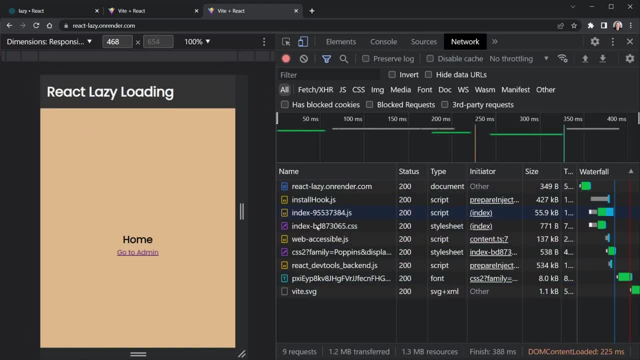 and i do that and we get these chunks of javascript. we don't get all the things we were before and you can see, here we've got like 55.9 kilobytes, and that's after it is zipped, or g-zipped, actually, because before it says resource size and i don't know if you can see that, but it was 165. 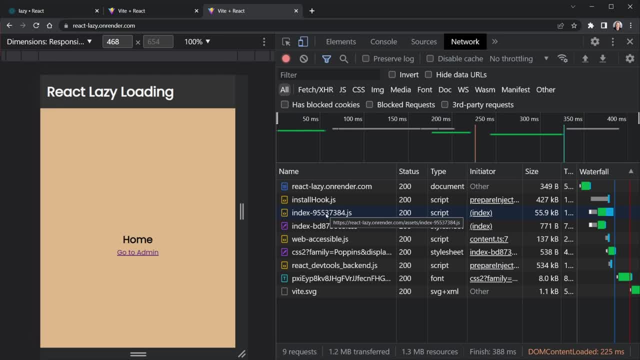 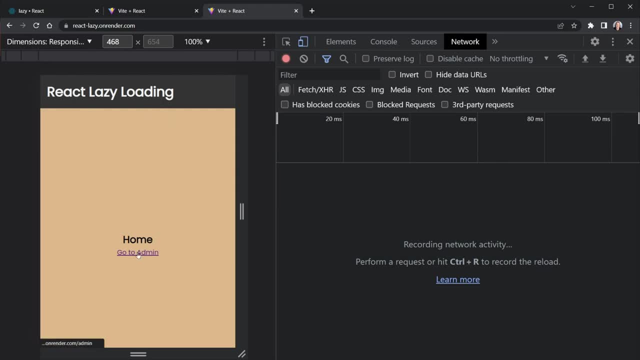 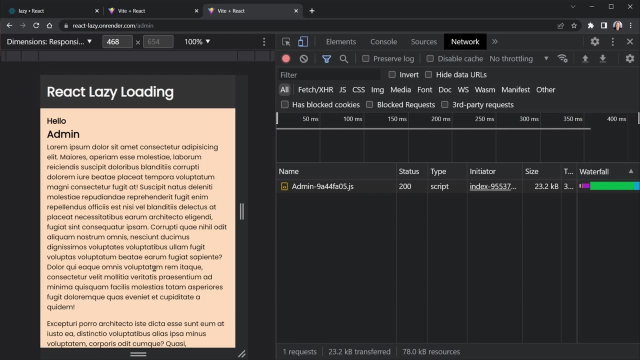 kilobytes, but that's not all. so now, if we were to go ahead, i can clear this out actually, so we can see what happens. we go ahead and go to the react lazy loading admin page, go there and look, we saw the suspense. we saw that, uh, skeleton loader for just a little bit and then we loaded some more. 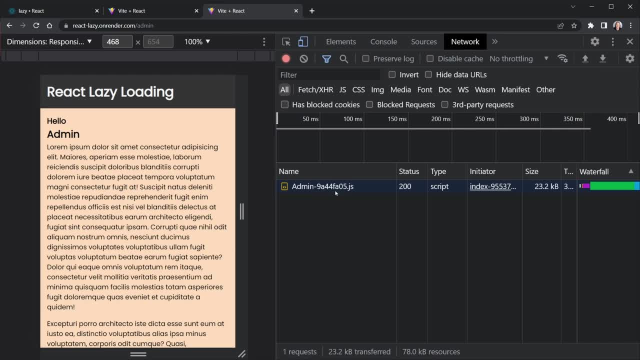 js. that's actually labeled admin dash and it has some numbers and letters over here as well: 23.2 kilobytes and i don't know if you can see the full resource size before that, but it's actually size before zipped was 78 kilobytes, so we really waited here. let's look at this time as well, that. 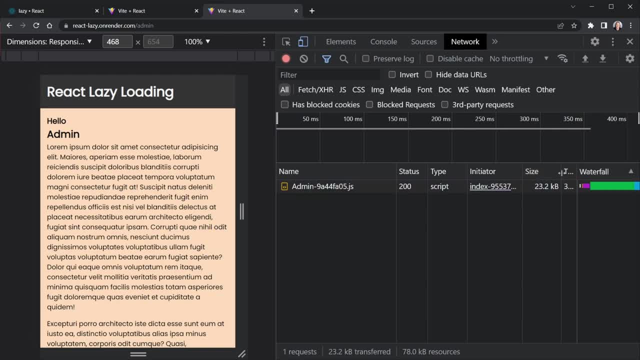 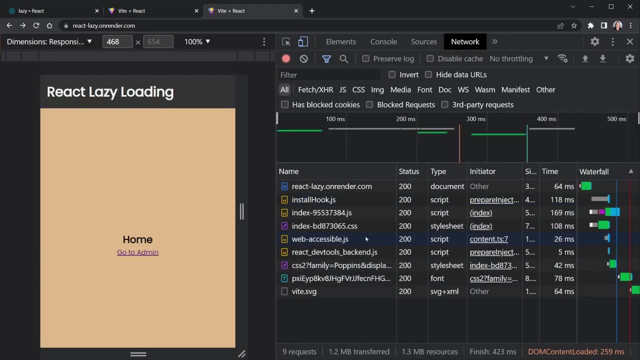 we see in the network tab. if i can pull that over now, we can see the rest of the time. 354 milliseconds. now let's go ahead and throttle this. let me go back and we let me do a empty cache and hard reload once again so it doesn't cache anything, or we wouldn't have to wait every time. now let's go. 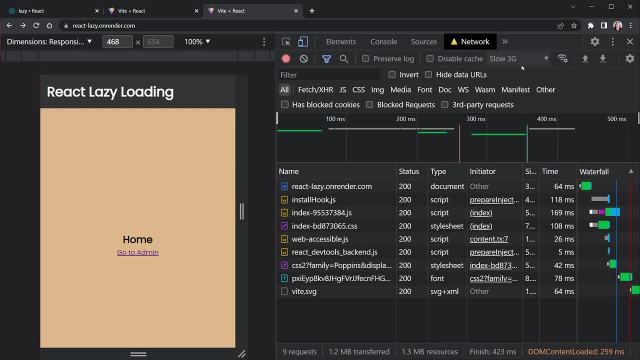 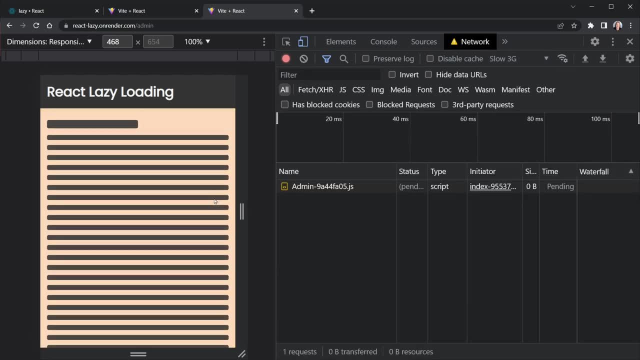 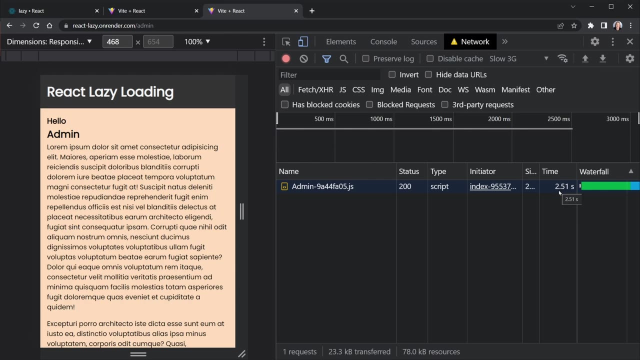 in here. let's do the slow 3g throttling that we can in the network tab, and i'll clear this out. and now let's go to the admin page. we should see this suspense loader, the, the skeleton loader, a little bit longer, and now it took two and a half seconds, not 350 milliseconds, but two and a half.